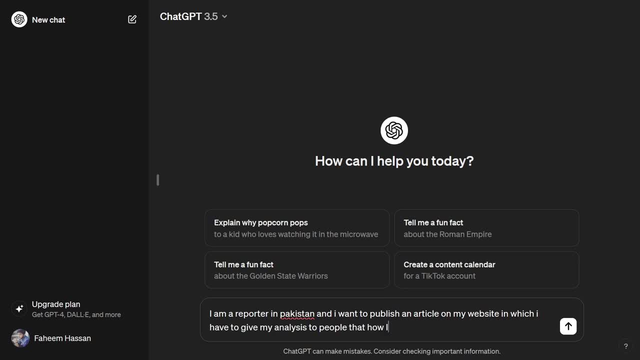 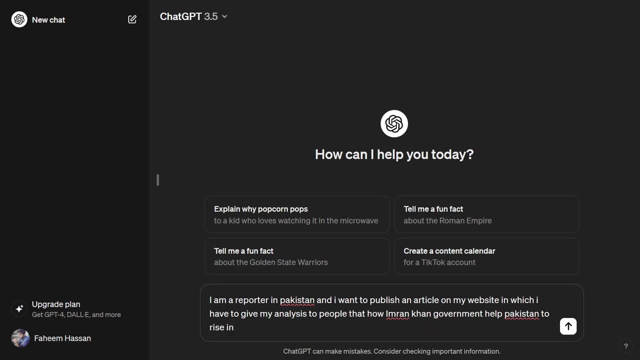 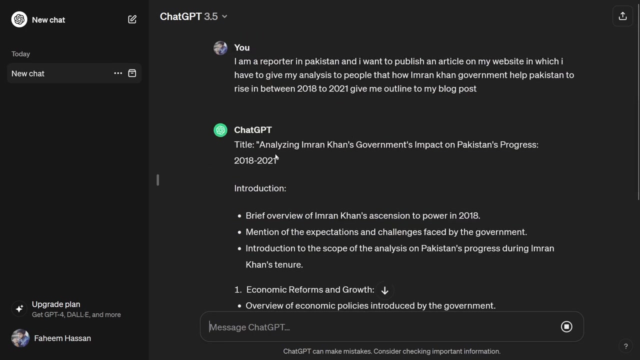 analysis to peoples that how Imran Khan government helped pakistan to rise in between 2018- 2021.. Give me an outline on my blog post. Let me press ENTER So you can see. first of all, it has given me a titles Like: 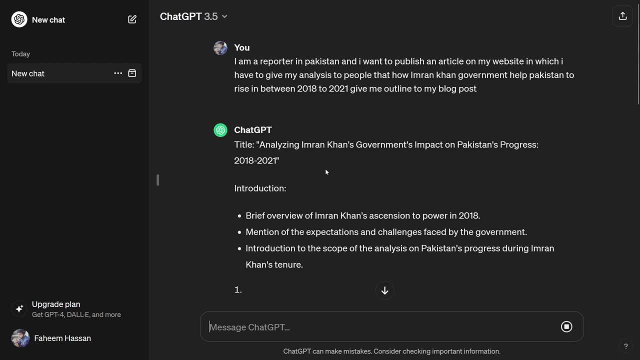 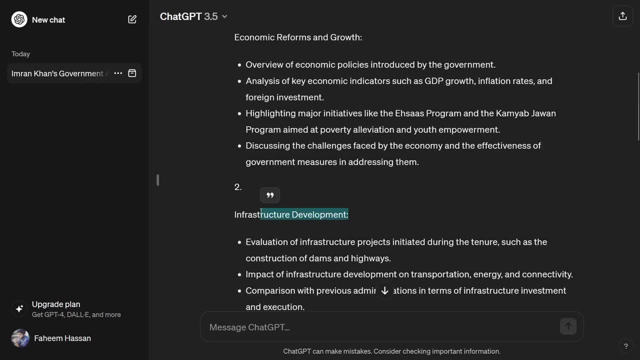 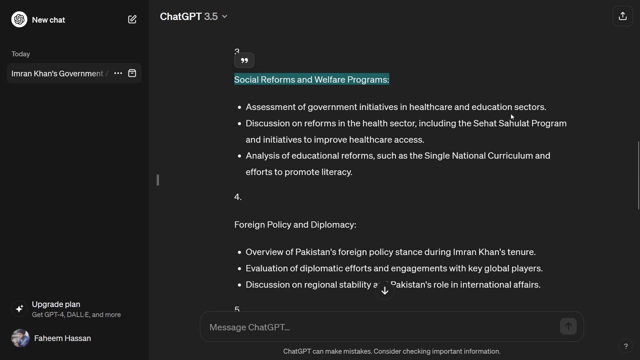 analyzing imran khan's government's impact on pakistan's progress 2018 and 2021: introduction, economic reforms and growth. infrastructure development and social reforms and welfare programs. assessment of government initiatives in health care and education sectors. discussion on reforms in the health sector, including the saith sahul program and initiatives to improve health. 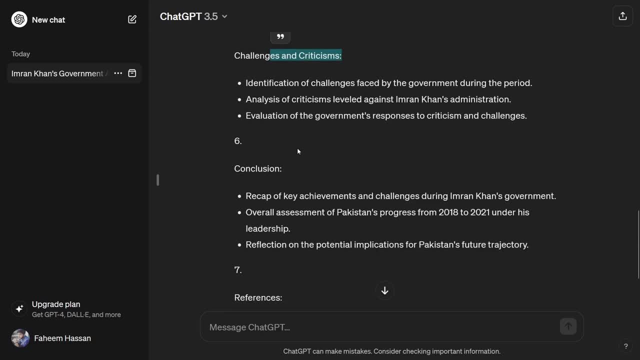 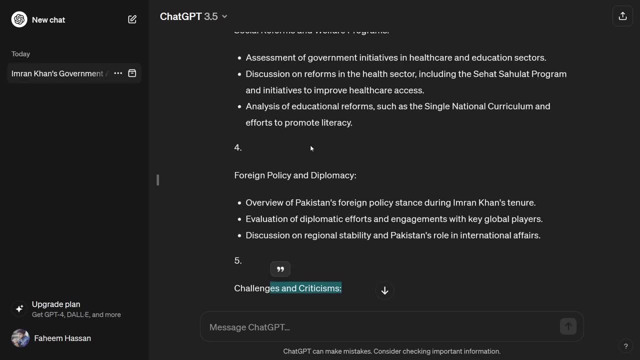 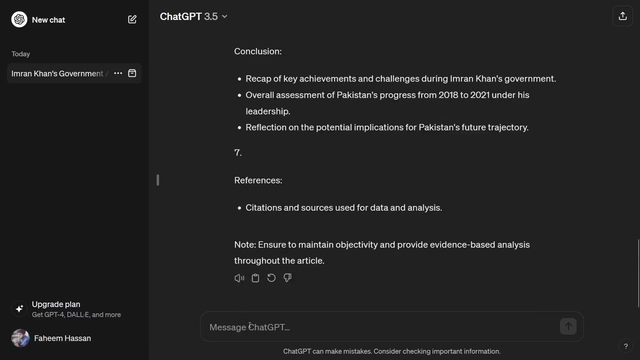 care access. so, as you can see that challenges and criticism, conclusion and reference, all these outlines are available for me. obviously this is very helpful. for example, i'm writing on this point like saith sahul program. let me copy this and here i'm going to type: here: give me detail. 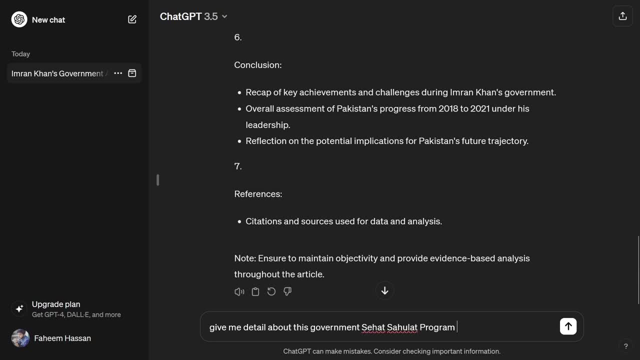 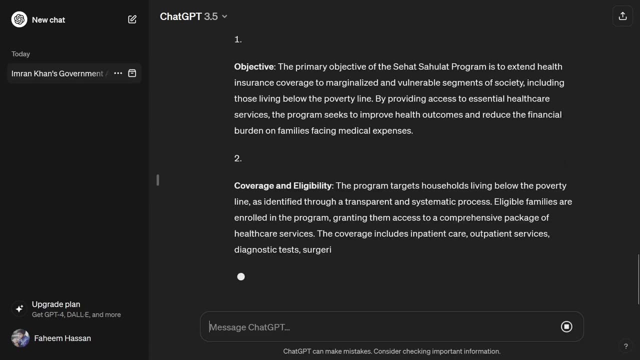 about this government, saith sahul program. let me press enter so that's how i can respond to this question. so i'm writing on this point like saith sahul program. let me press enter more and more and more on a specific topic. obviously you can- also you should get help from 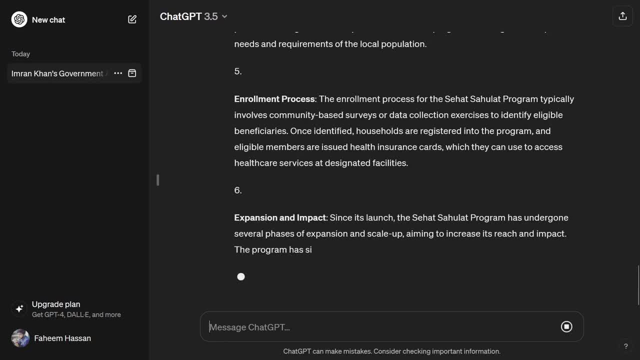 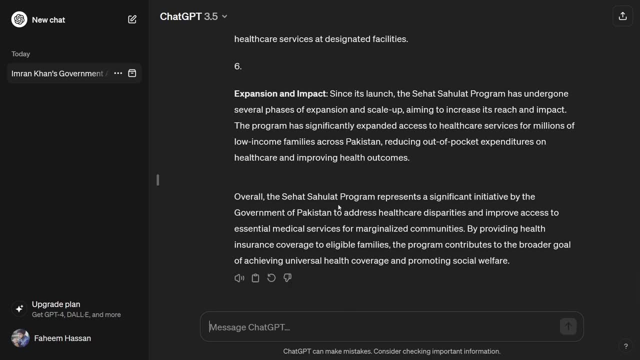 books, uh, from other newspapers, news channels, but these ai tools will also help you to write very effective content. now it's up to you. it is up to it is up to your creativity that how you get help from these ai tools. now, for example, uh, let me ask, we will ask chat gpd to assist us to use this. 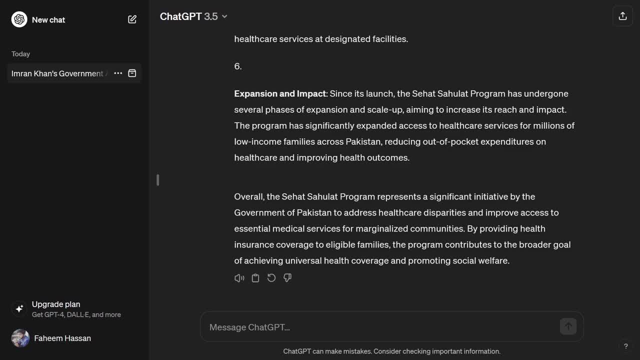 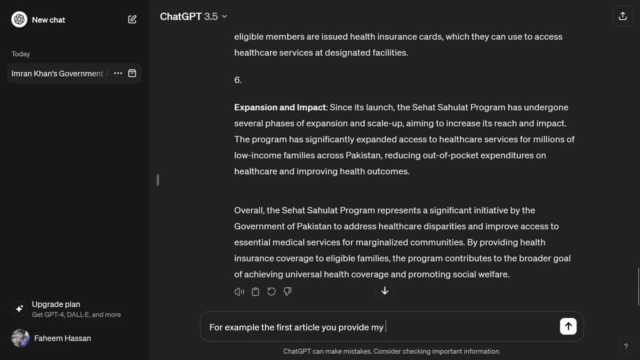 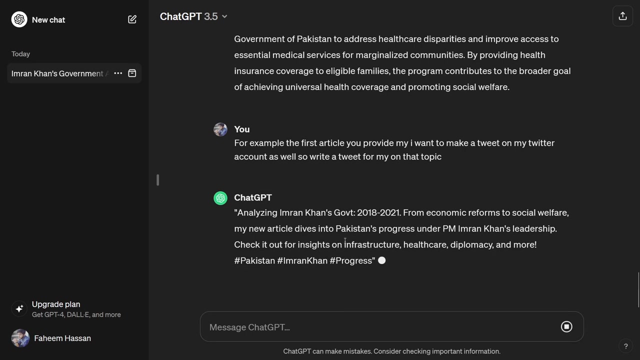 content to create engaging, promotional tweets for myself. okay, let me type here, for example, the first article you provide me. i want to make a tweet on my twitter account as well, so write a tweet for me on that topic, obviously. so here you can see that: analyzing imran's government from 2018 to.